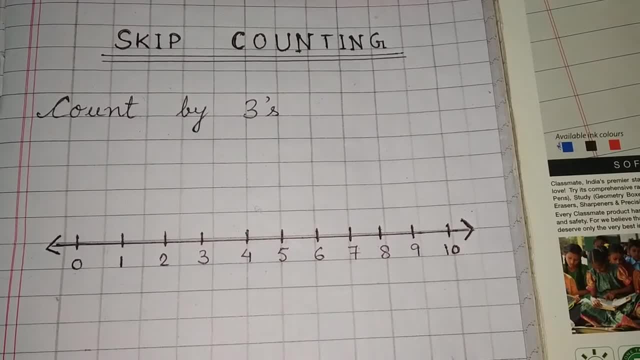 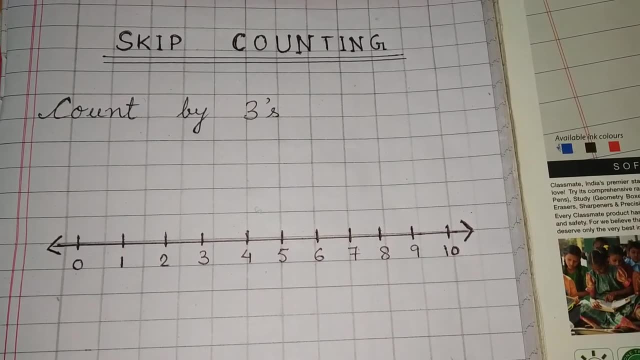 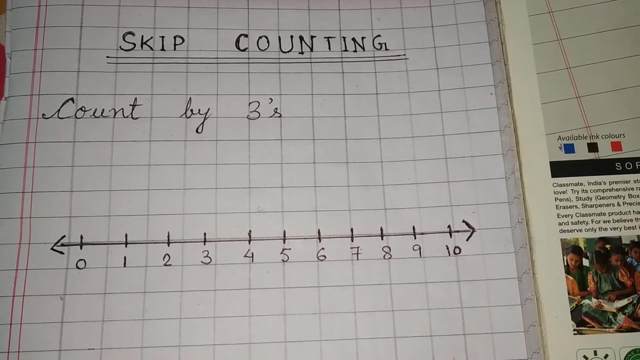 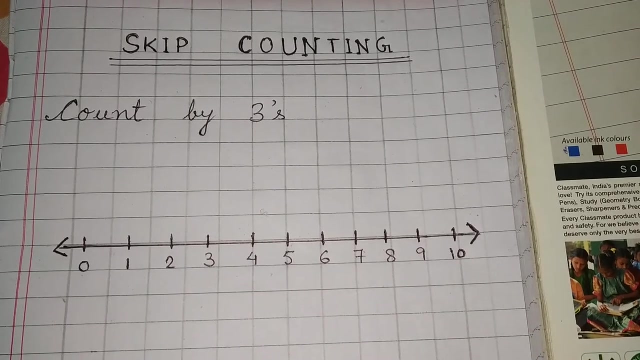 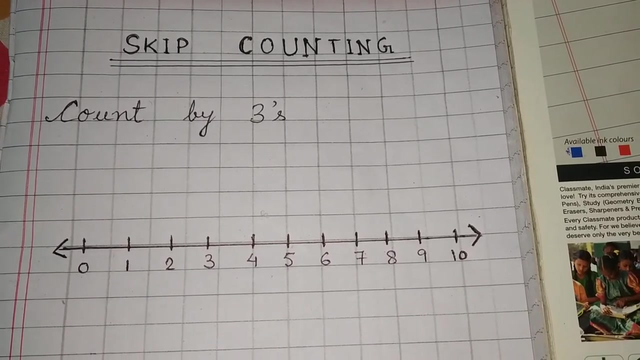 Good morning students. How are you all? I hope you all are fine. Today's topic in maths class will be skip counting by 3.. In my last video we have already completed skip counting by 2.. Now today we will be doing skip counting by the number 3.. 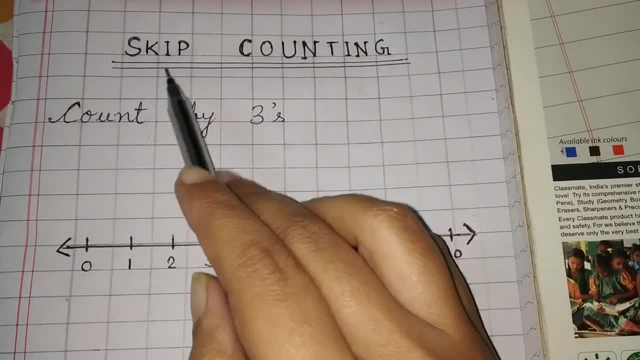 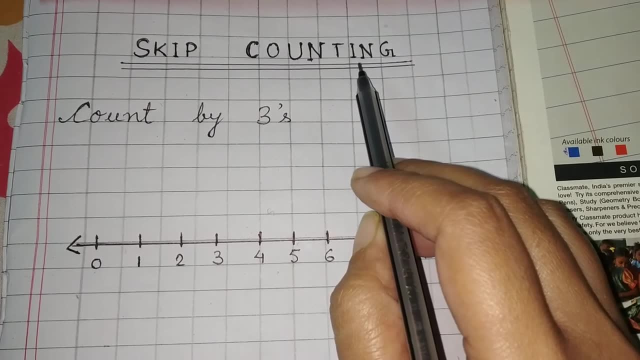 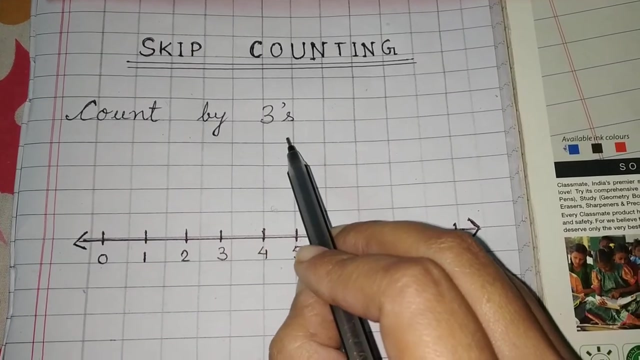 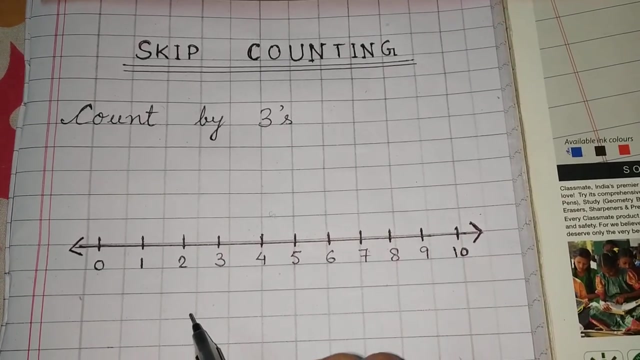 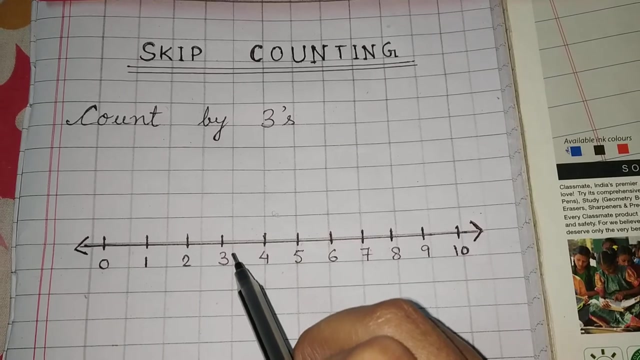 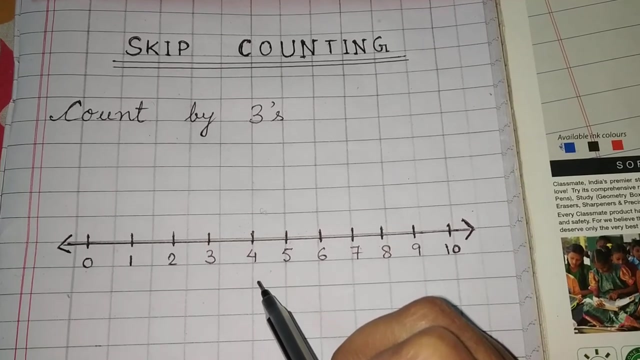 So, as you can see, here it is written skip counting by 3's. Now in today's class we will be doing skip counting, Skip counting by 3, that means we have to jump from 0 to 3 and again from 3 we have to count 1,, 2,, 3 and like this we will do the skip counting by 3.. 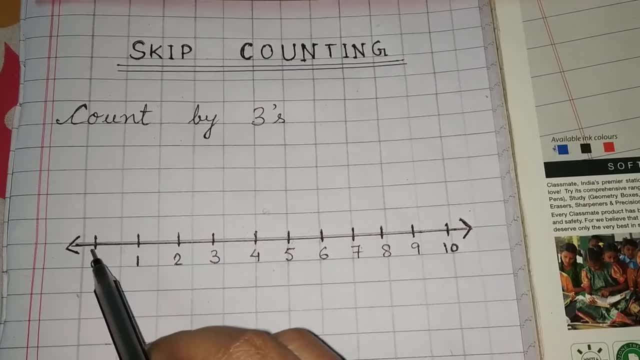 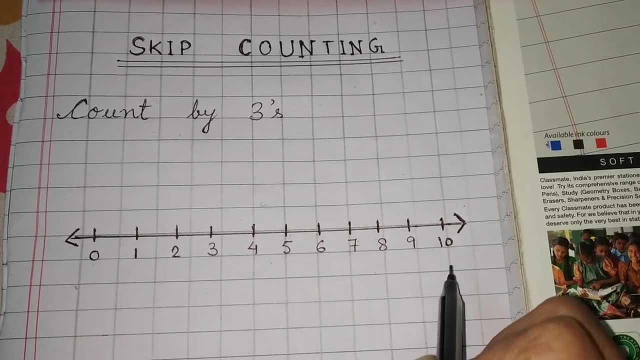 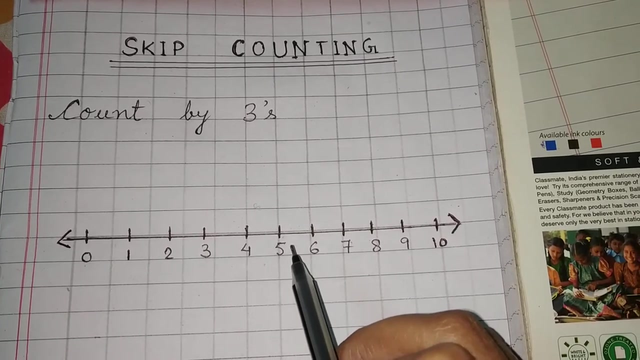 Now see how I am doing. As you can see here, I have drawn the number line which starts from number 0 to 10.. 0.. 1,, 2,, 3,, 4,, 5,, 6,, 7,, 8,, 9 and 10.. 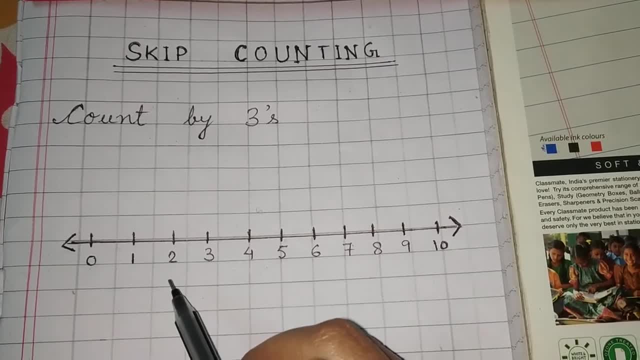 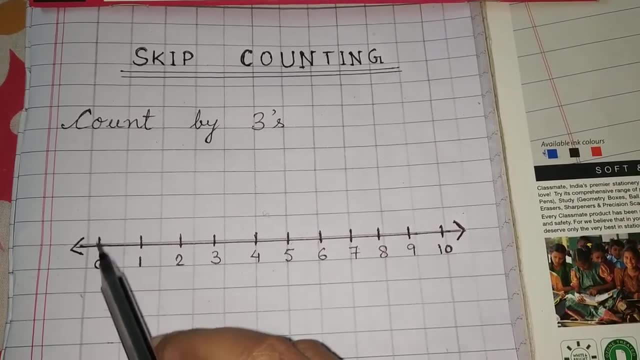 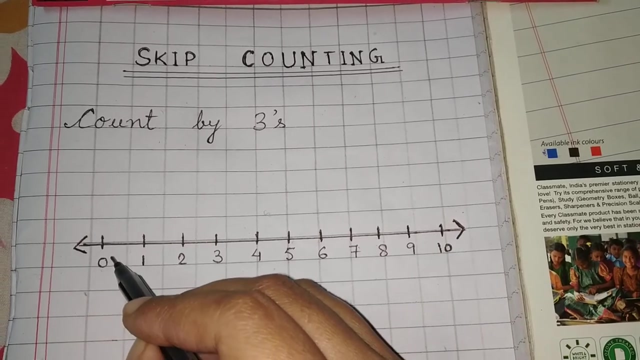 So now follow the students the way I am doing: count by 3's. So the first number is 0.. 1,, 2, 3.. We will draw a half circle from number 0. To number 3, because it is skip counting by 3.. 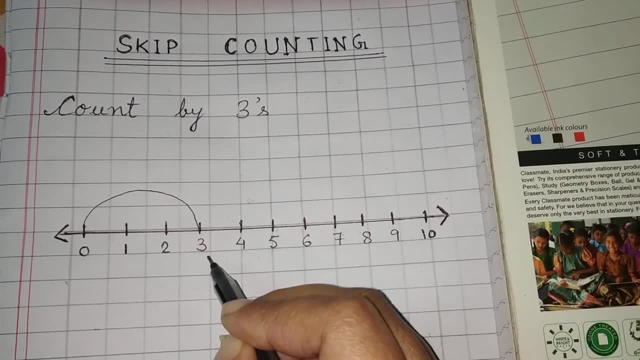 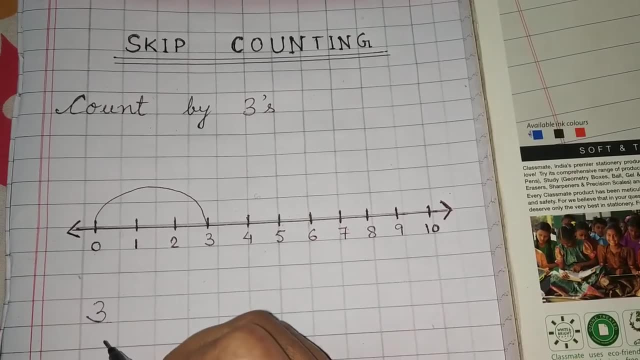 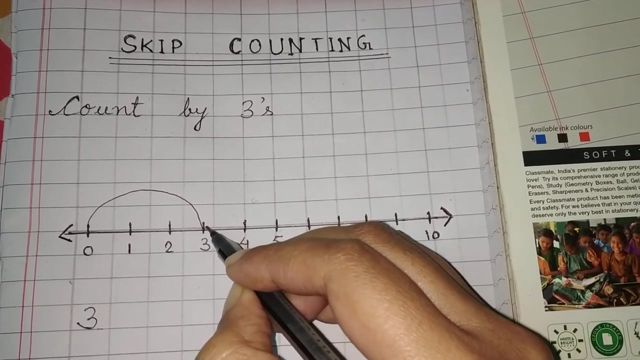 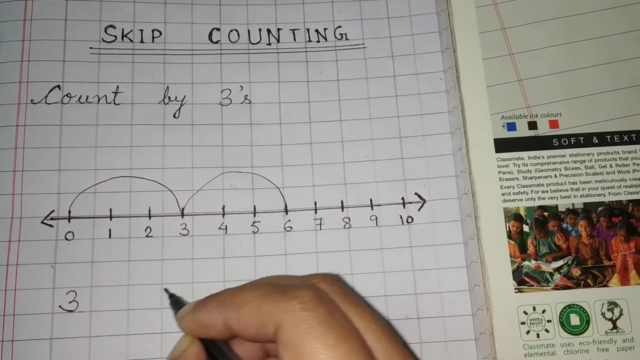 So the first number which comes in, skip counting by 3 is the number 3.. We will write number 3 here. Next 1, 2, 3.. So the next is 6.. So we will write here 6..